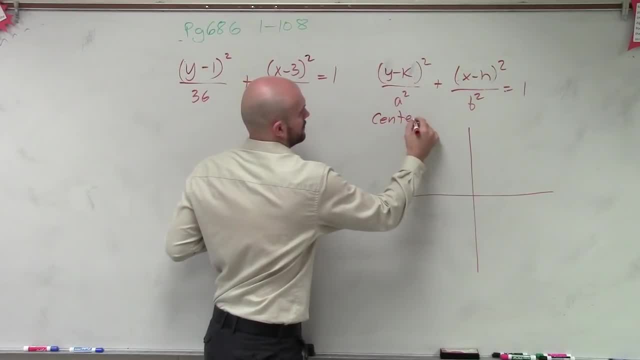 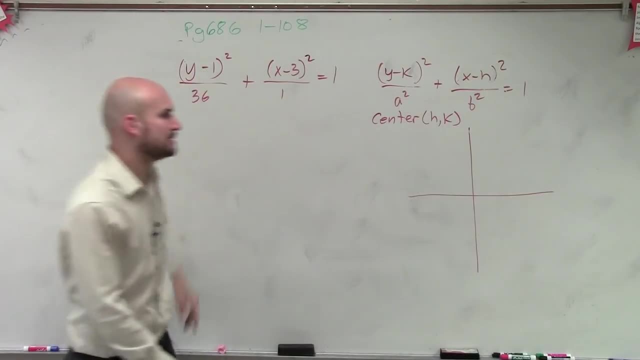 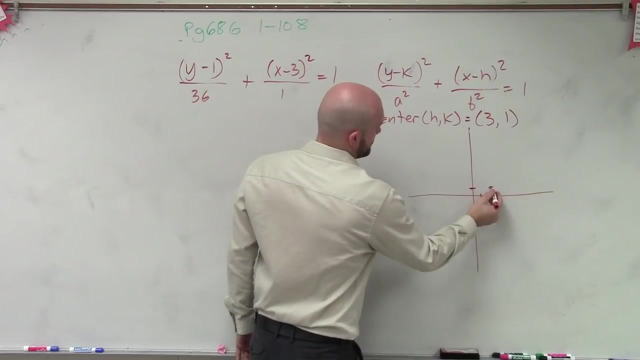 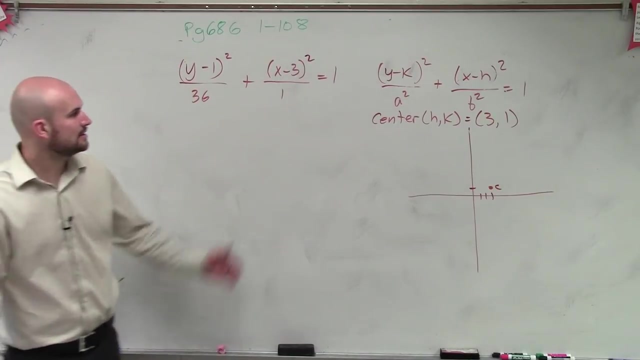 center is H comma K. So in this case, when you look at your formula, H is three, K is one, Because, remember, it's always the opposite. So let's go over three: one, two, three up one. So now I've found my center. Now we need to determine our vertices. All right, So let's go. 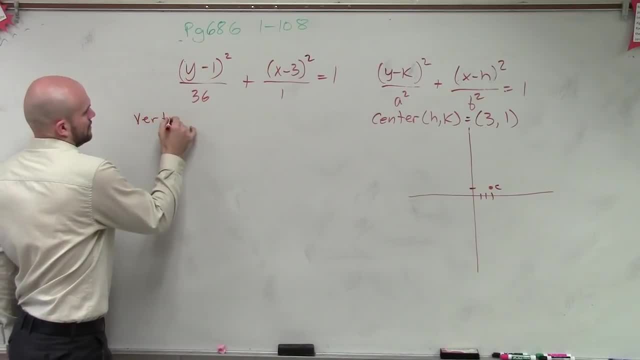 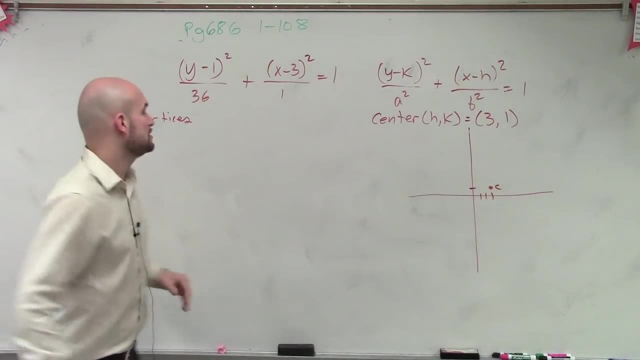 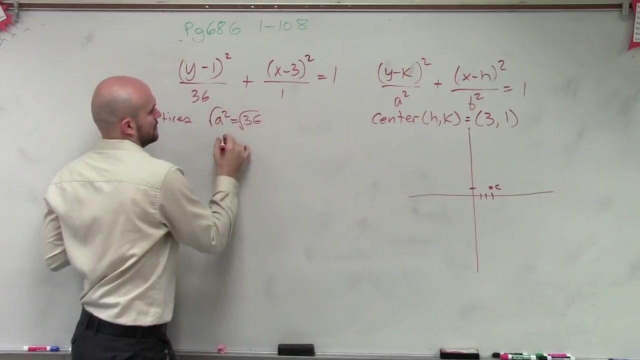 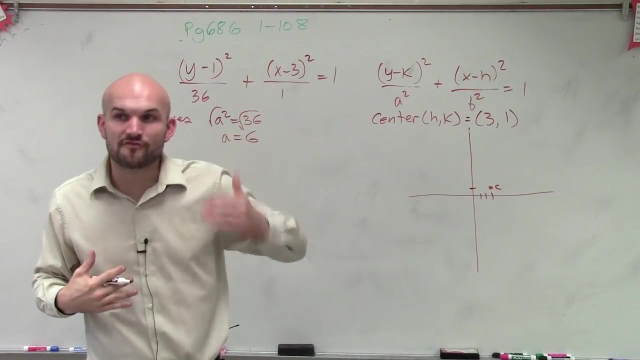 ahead and find the main vertices. So the vertices, remember, is going to be a distance of A right From the center. So if we know A squared equals 36, then we can say A, A equals six. Now, since we determined, ladies and gentlemen, that this was a vertical ellipse, are my vertices going to be? 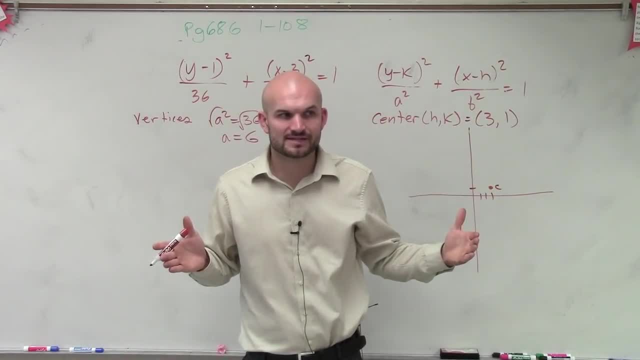 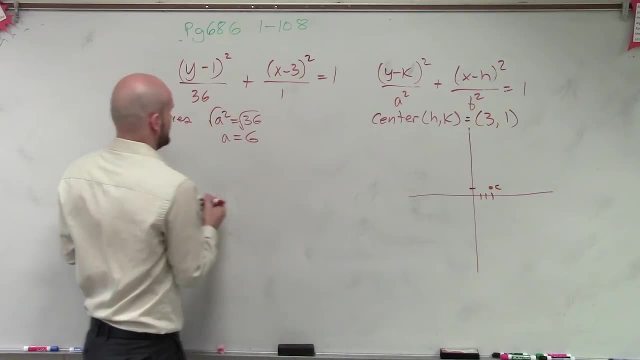 above and below the center or to the left. Well, they're going to be above and below the center, The left and to the right of the center, above and below right. So, to find my vertices, it's going to look like this: Your H is going to remain the same, but your vertices are now going to come in. 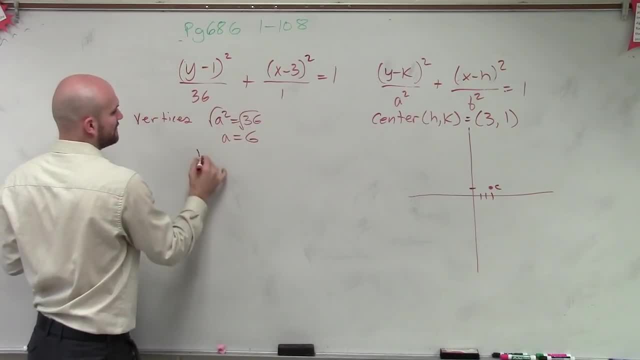 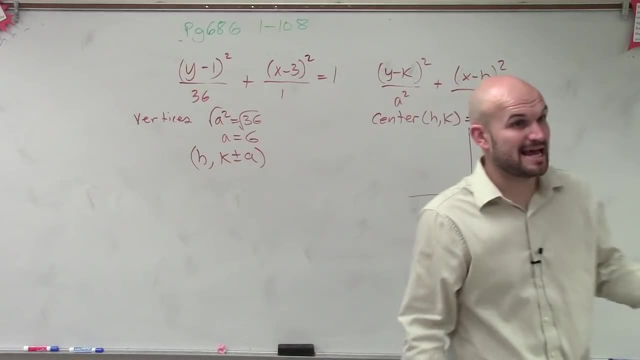 this form of this. So your vertices takes a general form of H comma K plus or minus A. So your H remains the same of your center right. Three is not going to change. but now what you're going to do is you're going to add your 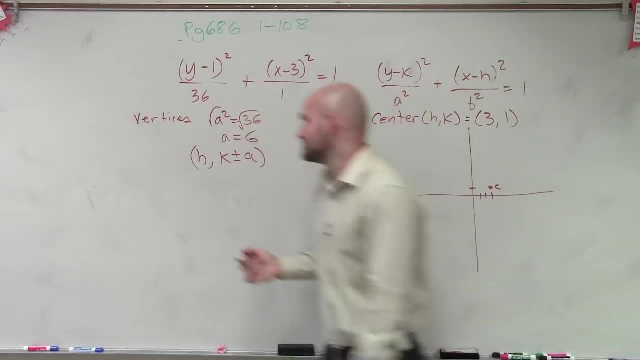 A to the K and you got to add or subtract it. So let's go and take a look at this. So my H is three, right, And my K? I'm sorry, my H is three, My K is one plus or minus six. So therefore I'm going. 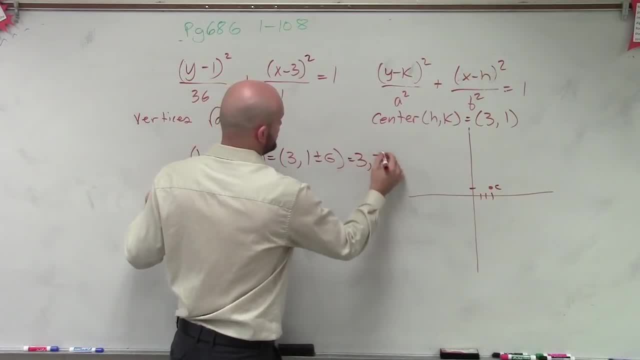 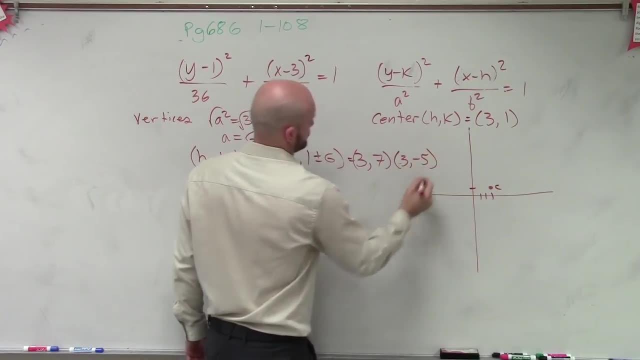 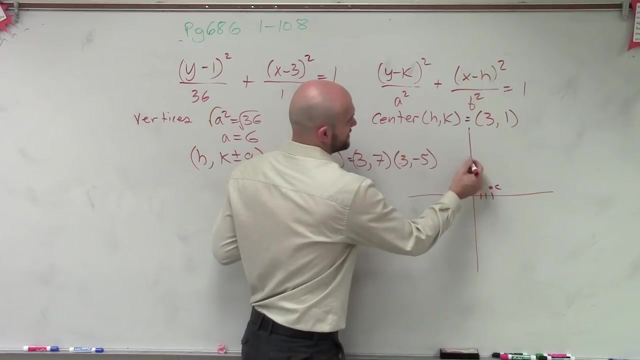 to have two vertices which are three comma seven and three comma negative five. All right, And let's look at that, Let's plot those points. So over three up seven, one, two, three, four, five, six, seven down five: one, one, two, three, four, five. 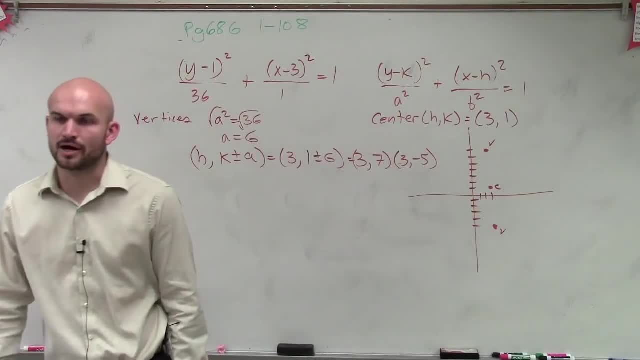 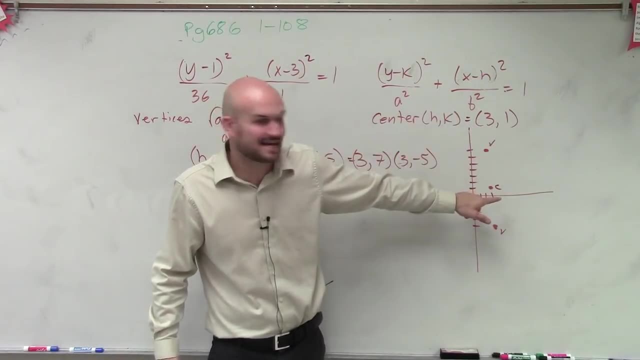 So what I've done is now just plotted my two vertices. All right, The other way you guys could do this is: you know that from the center to the next vertices is six units, right? So you could just go to the center and add six, one, two, three, four, five, six and you get to your vertices, or? 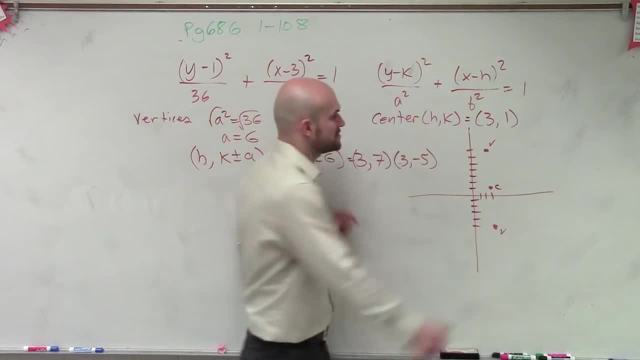 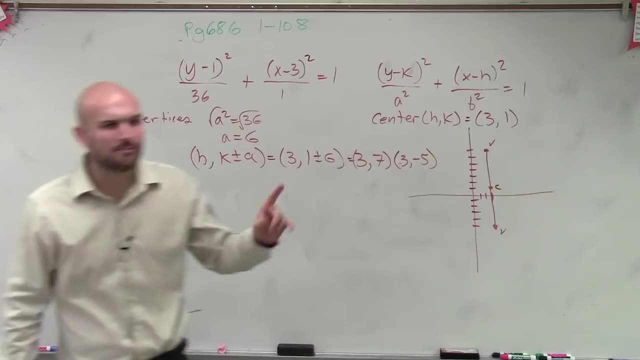 and then just subtract six, one, two, three, four, five, six. right Now, what we've just created is our major axis. Yes, Now there's one more thing that lies on that major axis. Anybody remember The foci right? We'll get to the foci here in just a second, though. 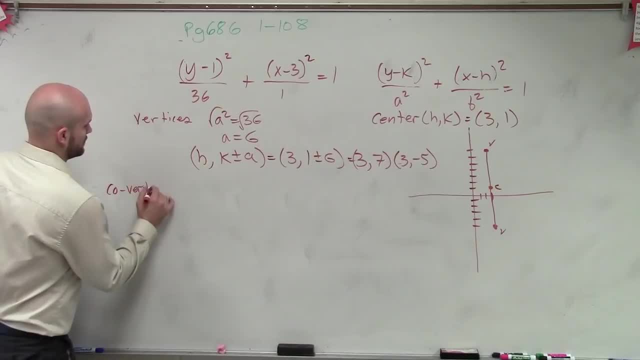 Let's go and determine now what the co-vertices are. So the co-vertices are your distance of B. So we know, B squared equals one. So therefore, B equals one. Now notice. the co-vertices, though, are now going to be. 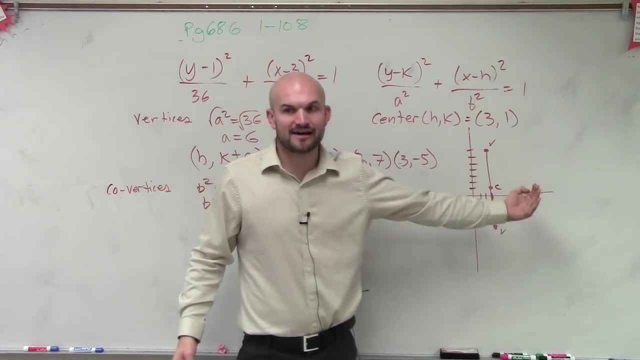 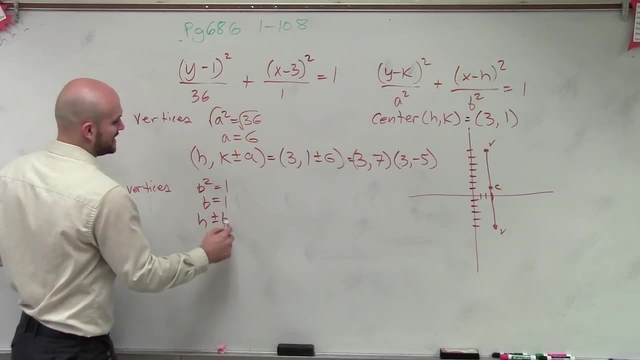 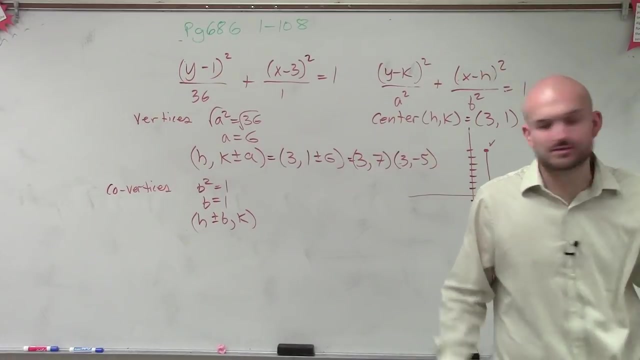 if your vertices are up and down, your co-vertices have to be left or right. So my co-vertices is going to be a little bit different. equation Now it's going to be H plus or minus B comma K, Because now the H coordinate on my center is that's where I'm going to be moving. So I'm 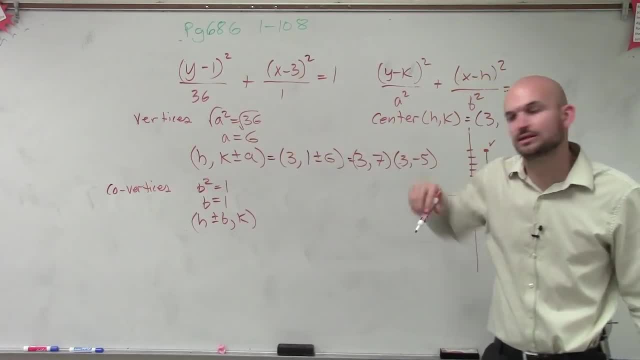 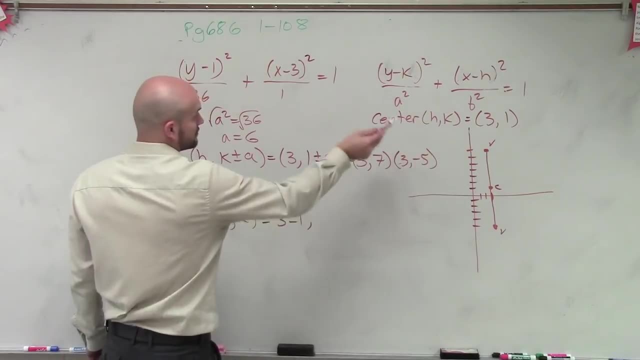 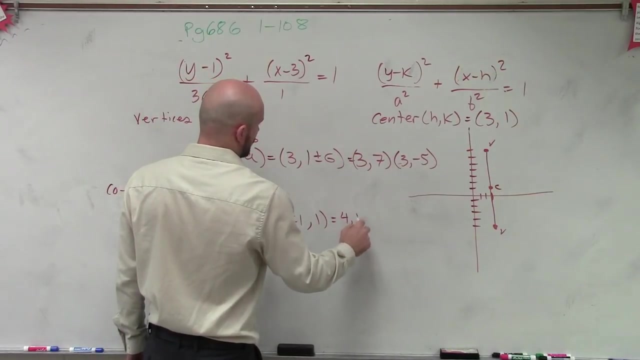 going to be moving one, shifting one to the right and shifting one to the left. But if you just want to look at algebraically, it looks like this: Three plus or minus one comma one. So that's going to give me coordinates of four comma one and two comma one. So let's plot those. 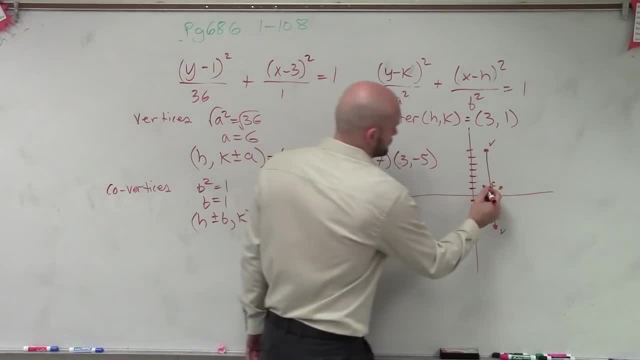 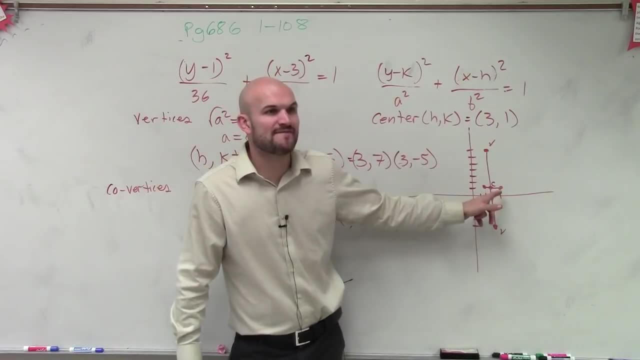 So those are going to be my two co-vertices, right? And you guys don't really need to do all this algebra work, Destin, because when you're looking at this you can just say, oh, my value of B. 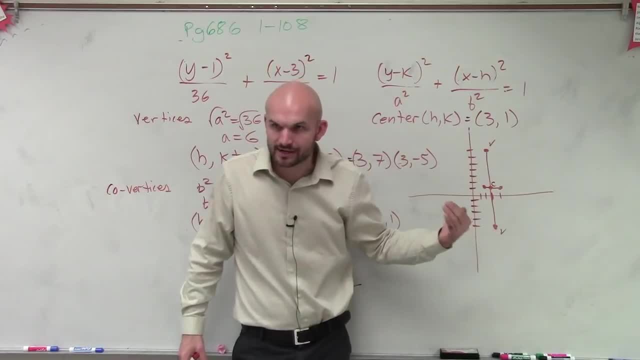 I'm just going to move it forward, I'm just going to move it backward. So that's going to give me a it from the center, one to the left and one to the right, correct? But then you guys can only see algebraic how we do this. Now we talked about our last. distance is our foci. 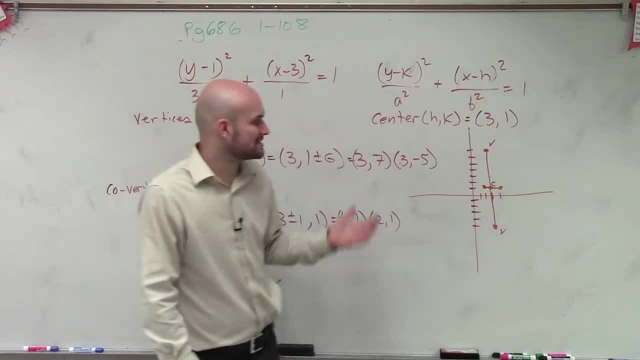 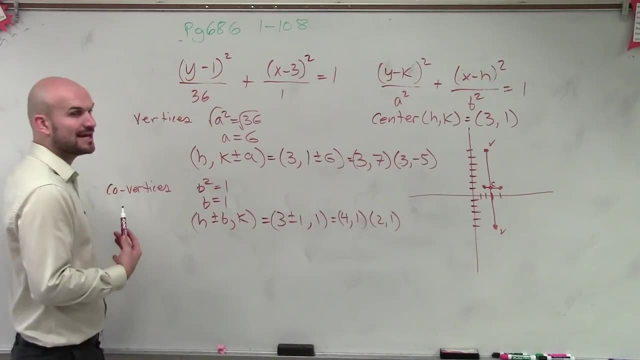 right, And the foci is going to be what? really? what's going to help us out? But remember, our foci is going to equal the C And we need to figure out what C is. So remember there is a relationship we talked about: A squared equals B squared plus C squared. That is the 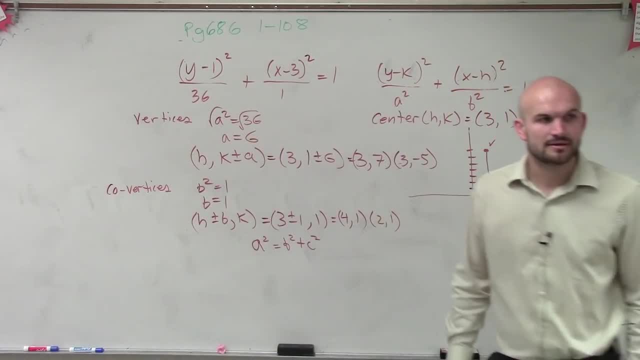 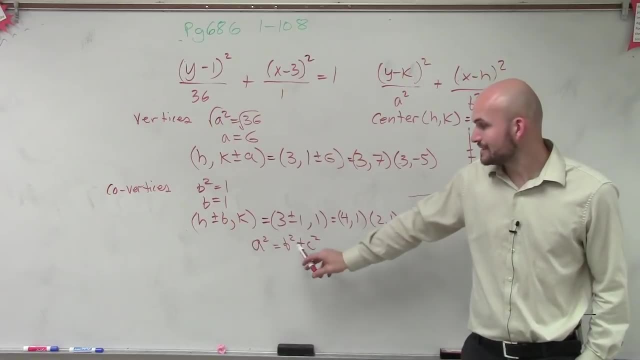 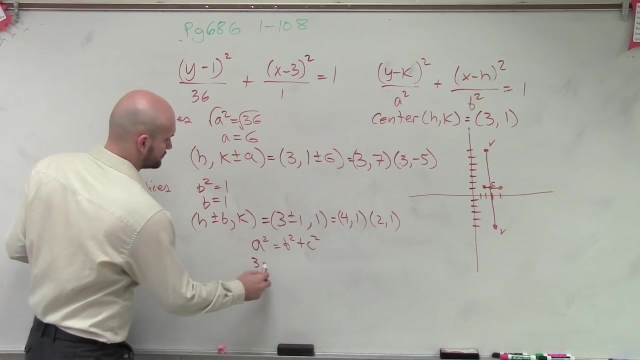 relationship of your distance A, B and C of an ellipse. And remember, C is the distance from your center to your foci. So now I need to solve for C. So therefore I know that A squared equals 36, which equals B squared, which is 1, plus C squared. So I subtract. 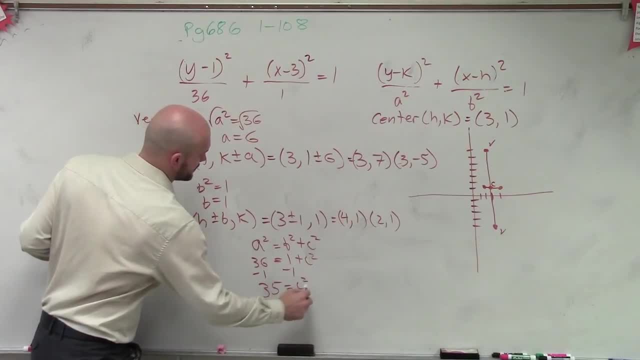 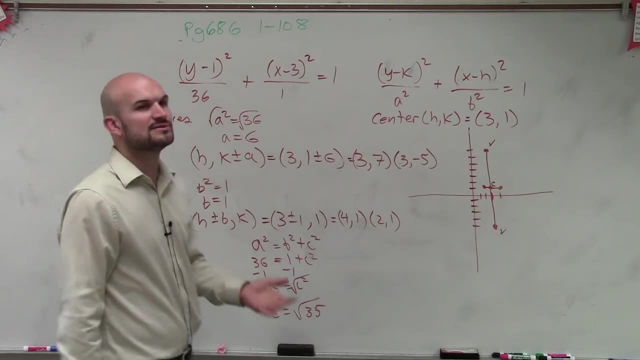 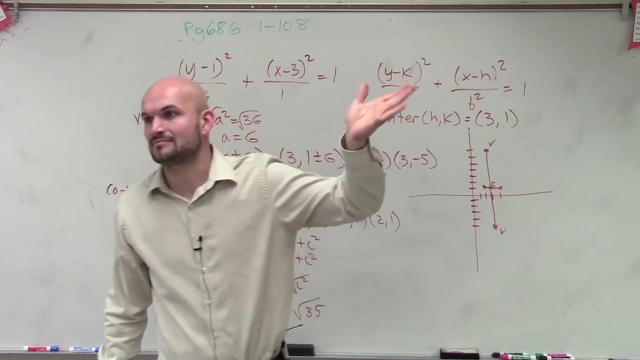 1, and I get: 35 equals C squared. Take the square root, take the square root. C squared equals the square root of 35. Now I can't reduce that, But if I give that a value that's going to be roughly like 5.89, something right around there. 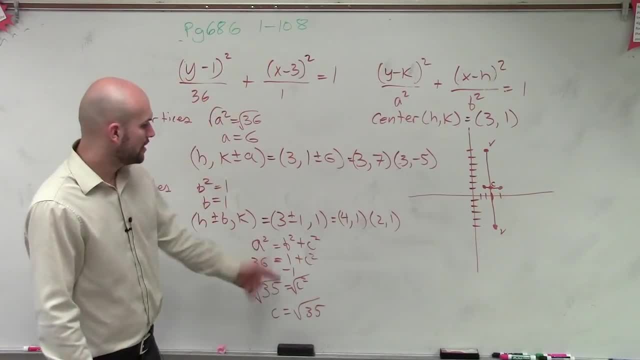 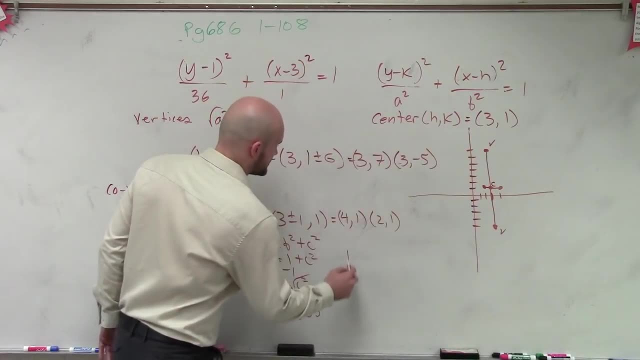 It's going to be high in the 8, 9 range, 5 point something. So what I'm going to do, though, is: where is that vertice? Remember, my foci have to lie on my major axis, So, anyways, just to kind of talk about the foci, 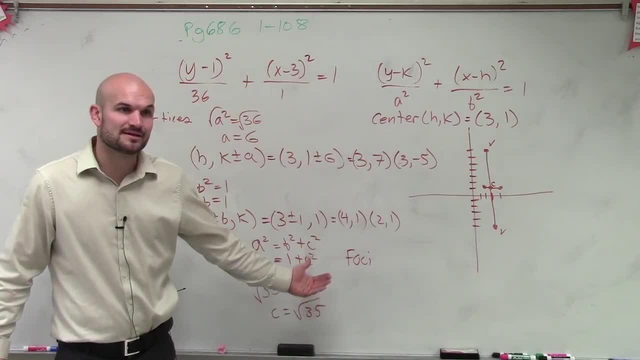 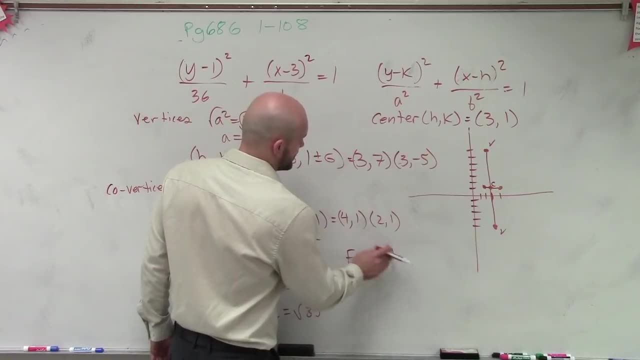 to give you guys the general formula. since this is a vertical ellipse, I'm going to be adding or subtracting the foci to my h-coordinate. So it's going to look something like this: to my k-coordinate, h comma k plus or minus c. 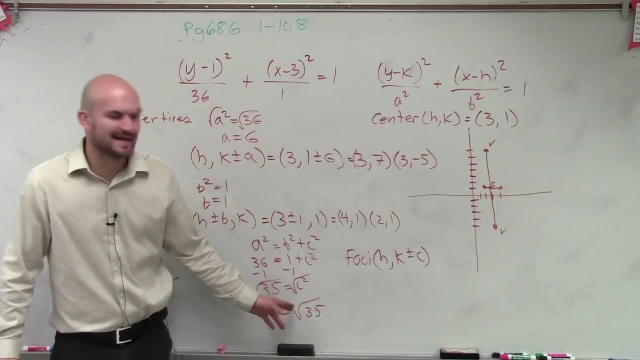 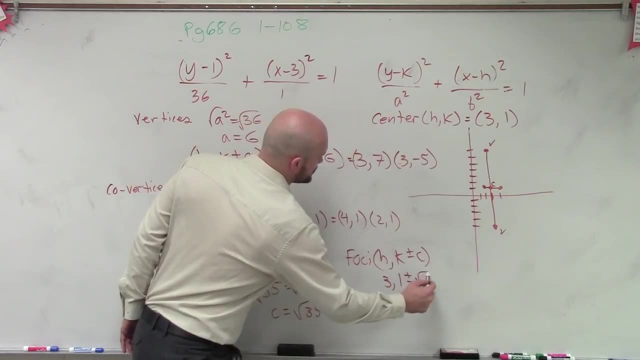 Now we're going to come into a little bit of a problem here, because we can't add the square root of 35 to my k coordinate. But anyways it'll look like this: 3 comma 1, plus or minus the square root of 35.. 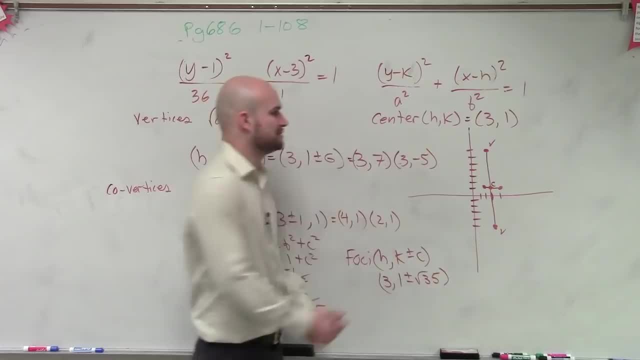 Now I can evaluate this. We could go to decimal And when you do, guys get the decimal form, you're going to see that it's going to be, your foci's are going to be like right next to your vertices. 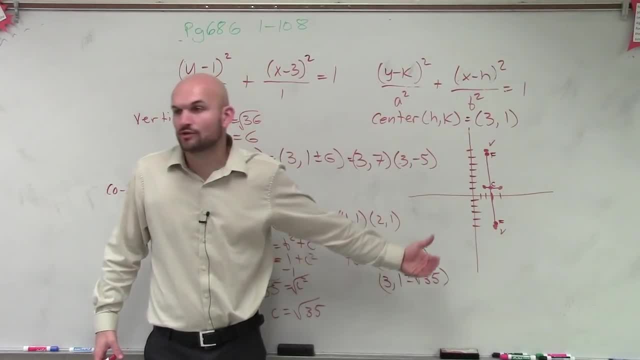 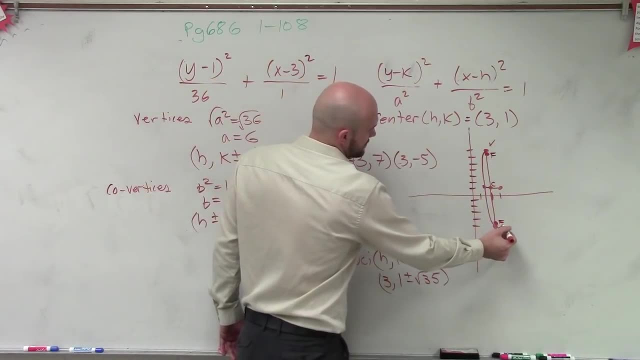 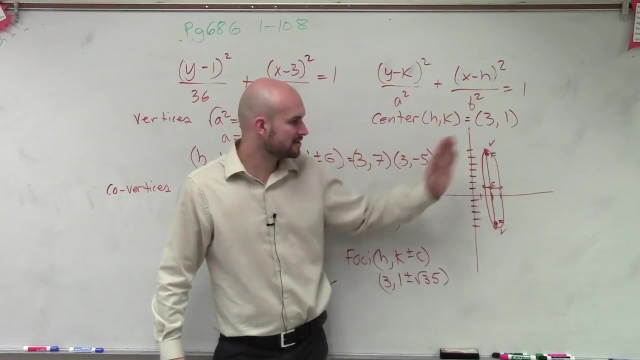 Because, as we talked about, the square root of 35 is 5.9 something. So now just to go and graph it, connect to my vertices and my co-vertices, and there it is. So now what I've done is showed you the center, the foci. 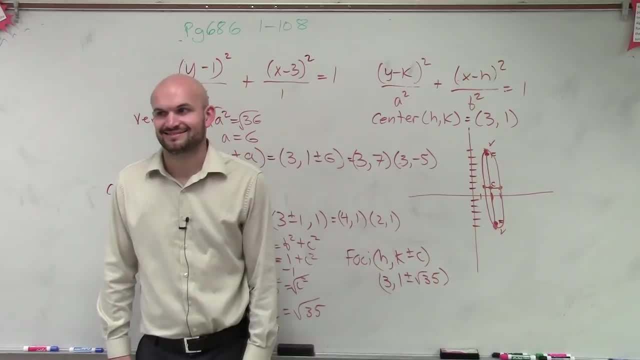 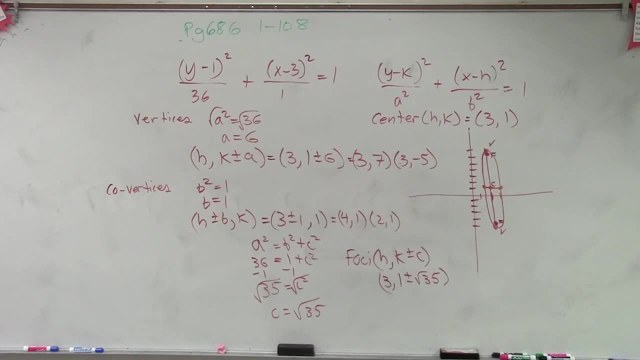 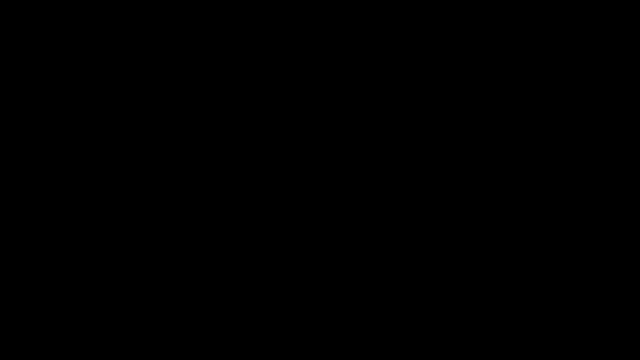 the vertices and the co-vertices, And we're going to thought about the co-vertices. Let's see if we can use this to compute this real fast. There we go. fancy Principle: Ass Wireless, SPEAKER 1 and SPEAKER 2.